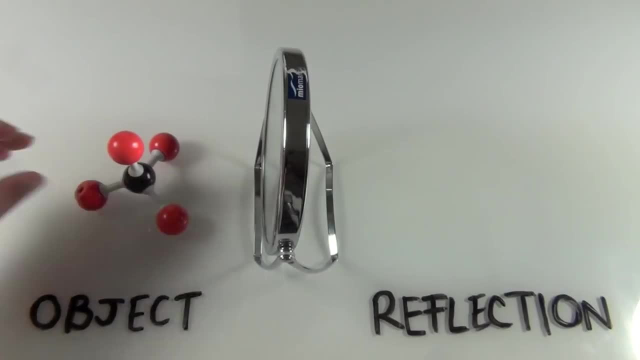 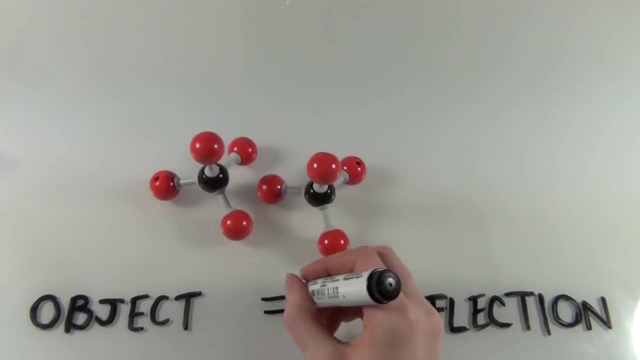 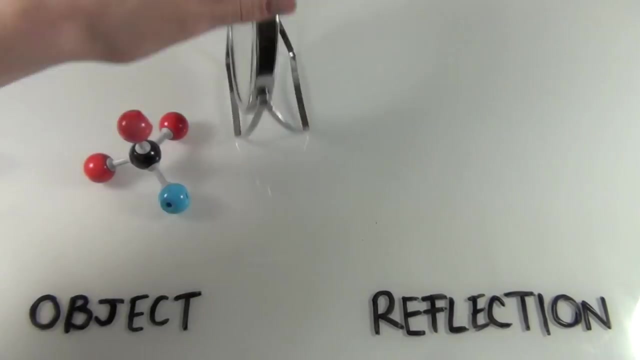 on to some kind of hypothetical molecule. We have the object and its reflection And again we can very easily see that the object is identical to its reflection. Now, changing one of the balls to blue, We ask again: is the object identical to its reflection? And the answer is yes, So changing. 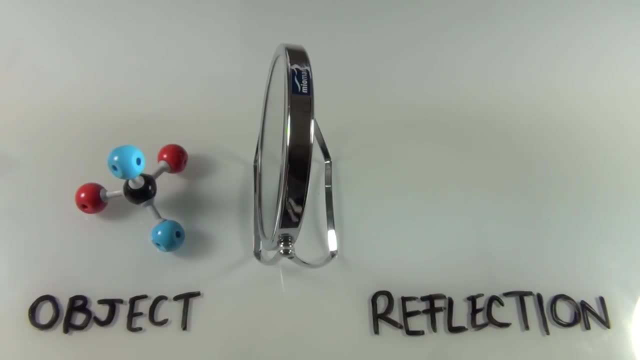 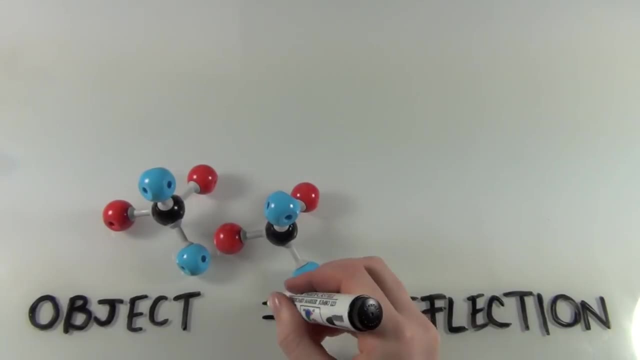 another of the balls to blue. We ask again: is the object identical to its reflection? And again, the answer is yes. Changing another of the balls to yellow And changing another of the ball to black, We ask again: is the object identical to its reflection? And the 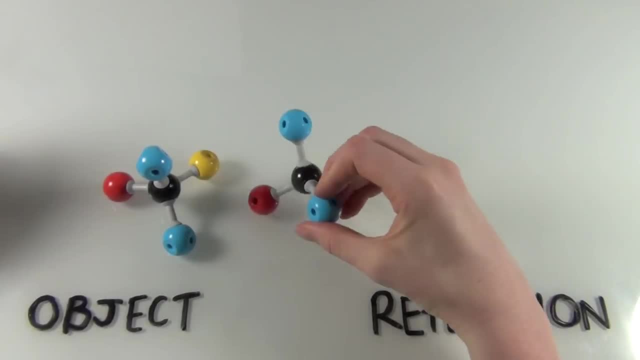 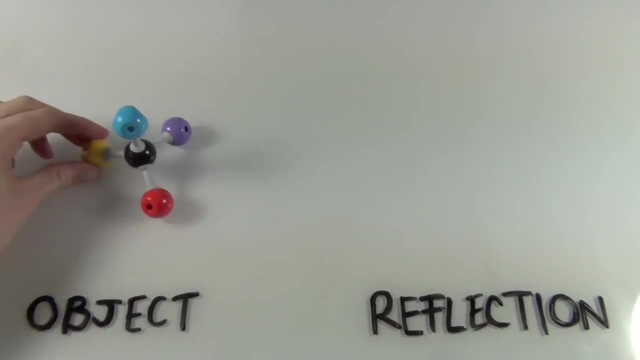 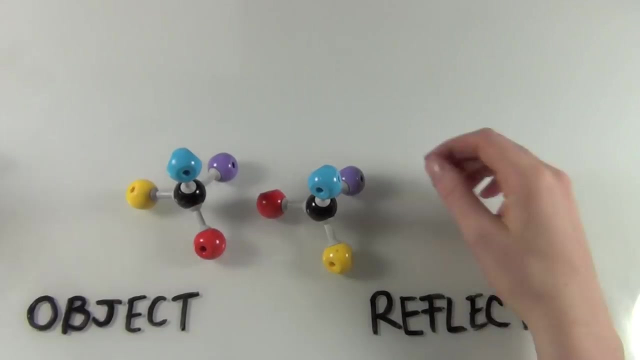 answer is yes. So changing one of the other balls to white And changing one of the other balls to red And changing one of the other balls to green And changing one of the other balls to red And changing one of the other balls to blue And changing one of the other balls to black And changing one of the other. 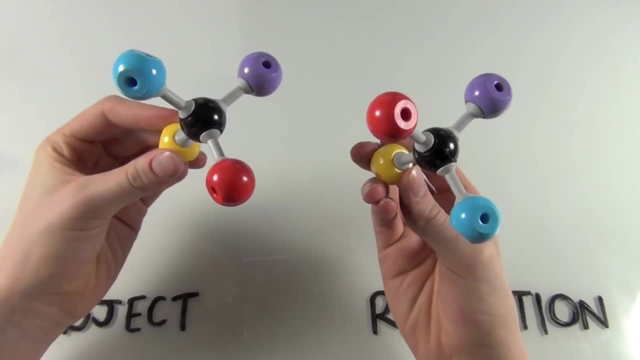 ones to yellow And changing one of the other balls to star, Andomposing them for previous root. Now we can use the süimpelemet and finish up our subtraction to read and evolve. And now we can dump the last star, Olivier, over in normal like this, And we can now busy CLICK. 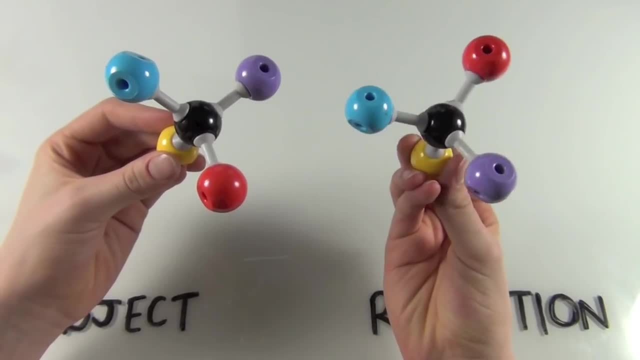 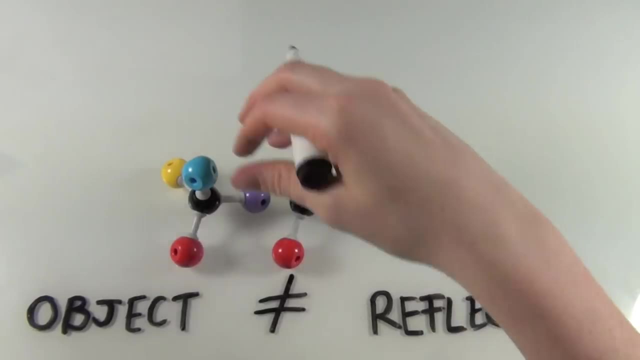 and actually repeat the process over and over again, And then simply keep the previous two, so that all the colours are in the same place. In other words, the object is not identical to its reflection, And this is what chirality is all about. 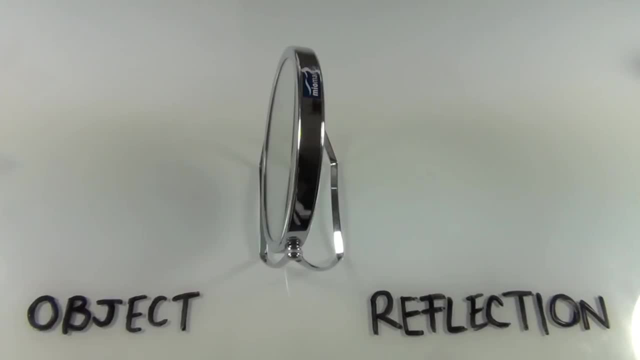 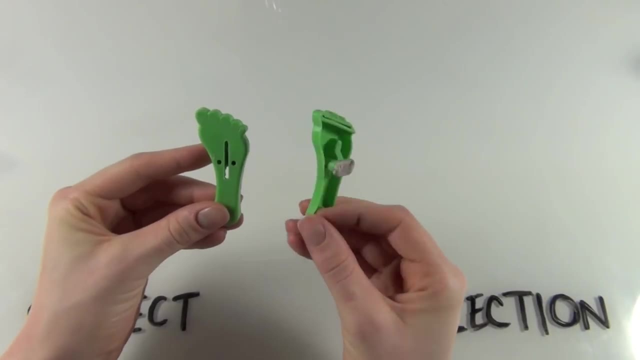 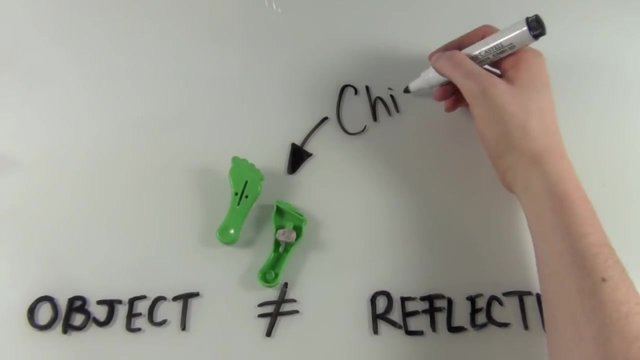 when the object is not identical to its reflection. So we have another object and its reflection And there's no way that I can rotate the reflection so that those two objects are the same, So they are chiral objects. Again, we have some made-up molecule. 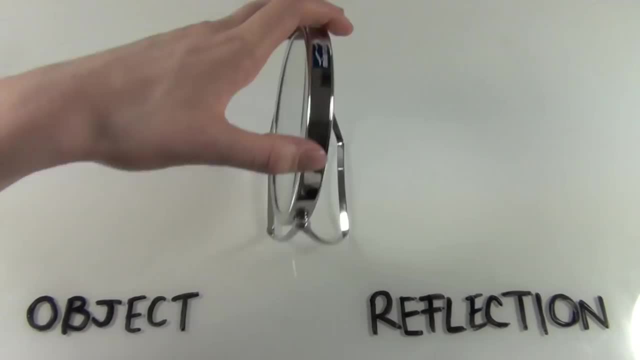 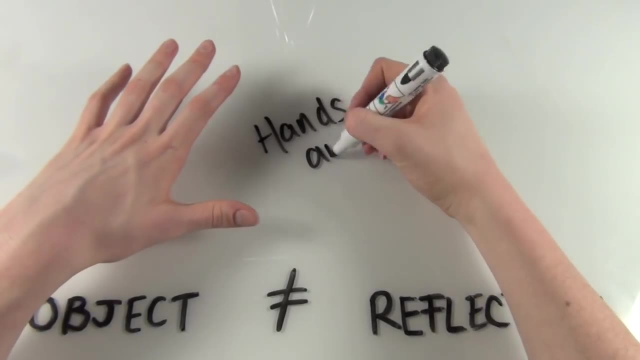 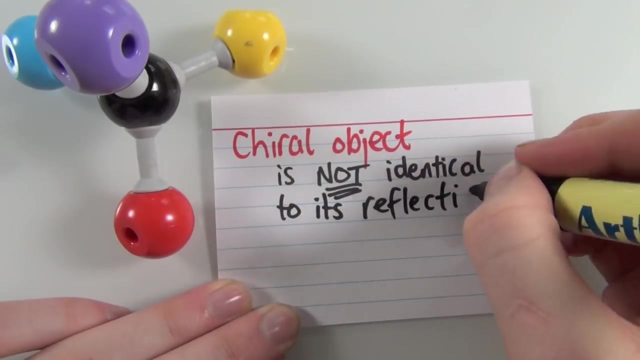 And this made-up molecule is achiral. And finally, we have the famous example of hands, And my left hand is not the same as my right hand, which makes my hands chiral. So, to sum up, a chiral object is not identical to its reflection. 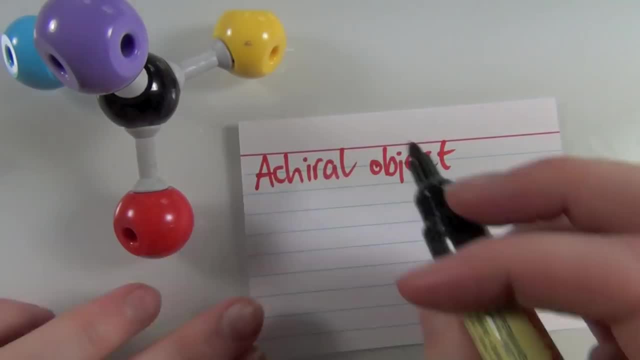 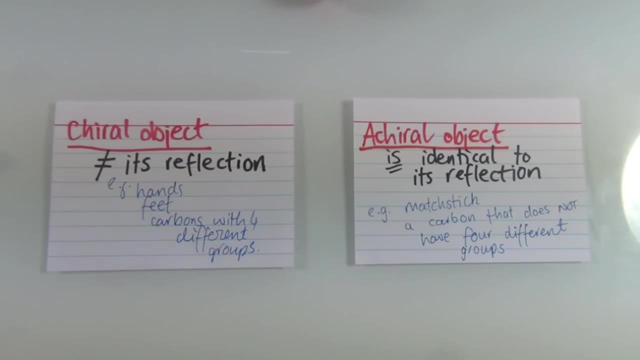 And it's not identical to its reflection, And an achiral object is identical to its reflection. Okay, so I hope you now understand the difference between chiral and achiral objects. If you liked it, don't forget to subscribe, because I'm going to be making lots of biochem and neuro videos. over the next few months.